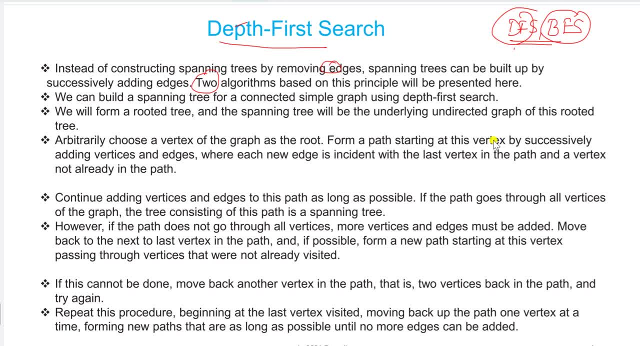 of this DFS and BFS. Now I am going to discuss about how we can connect to the trees with the help of depth first search. So in depth first search, remember the steps. First step would be: see here, find out. or, arbitrarily, you can choose the spanning tree for a connected simple graph using 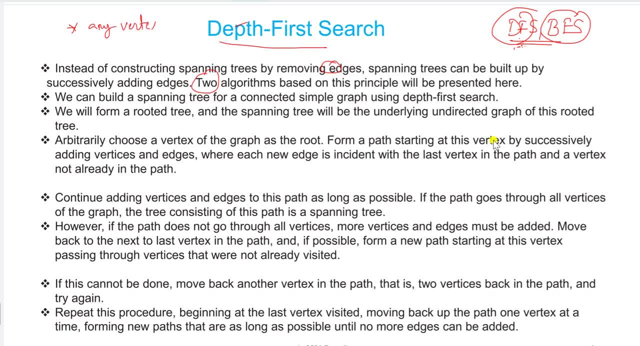 any vertex. you can choose any vertex in a particular graph. okay. So you can choose any vertex in a particular graph. In case in examination he mentioned: okay, in examination, if he mentioned like starting vertex will be A or starting vertex will be F, like this, then you have to choose that vertex only. okay, Otherwise you can choose any vertex in a particular graph. That is the point. Orbitally, you can choose any vertex of the graph as the root. 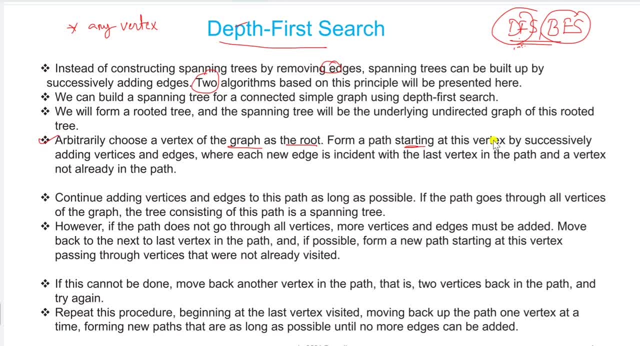 Okay, So, from the path starting at this vertex, by successively adding the vertices and edges where each new edge is incident with the last vertex in a path. okay, when there is a knot already in the path, In the second step, what we have to do means you choose some vertex called A. okay, So explore this vertex. How you can explore what are the adjacent vertices. 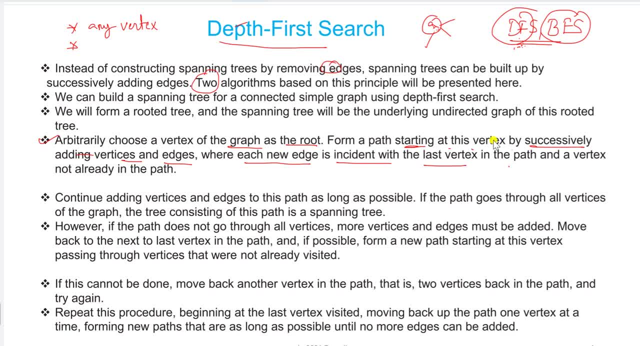 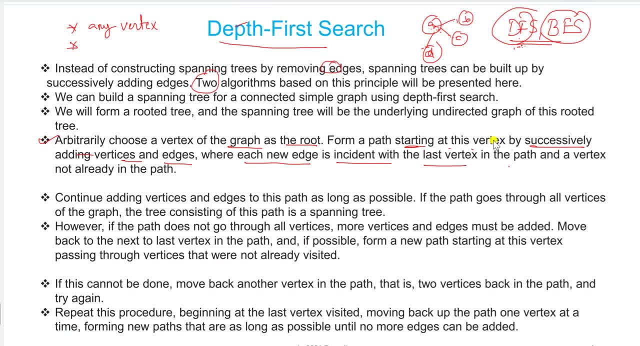 So A have all these three edges. You can choose, after A, any one of this, any one of this. For example, you choose C. okay, Now you are choosing the next vertex. vertex a, comma, c. okay, now you explore. c explore means what visiting the next incident. vertex in. 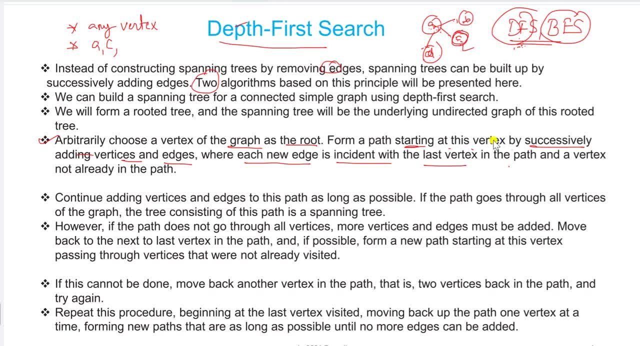 a particular graph, okay, and that should not be already in the path. for example, after c, here we have a, d and e. okay, so here c have two paths, ma. so d and e are there, right? you can choose any one, d and e- if it is not already existed. if it is not already existed, you can draw, you can. 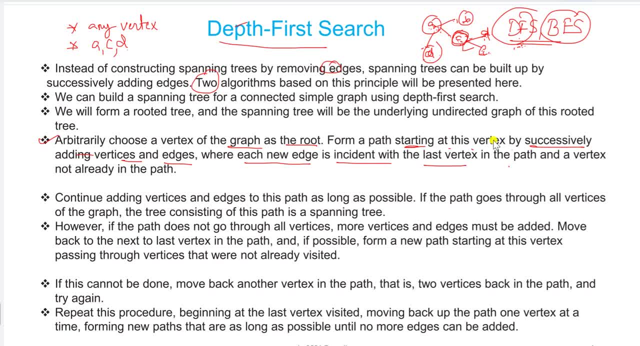 draw, if it is already existed, just backtracking to that particular vertex and do follow all the steps again and again until you reach or you visit all the vertices in a particular graph. these are the steps to find out the depth first, first search, first search, look, are them okay? here the thing is what the vertex that유라고 많이 CONTINUE TO FIND. 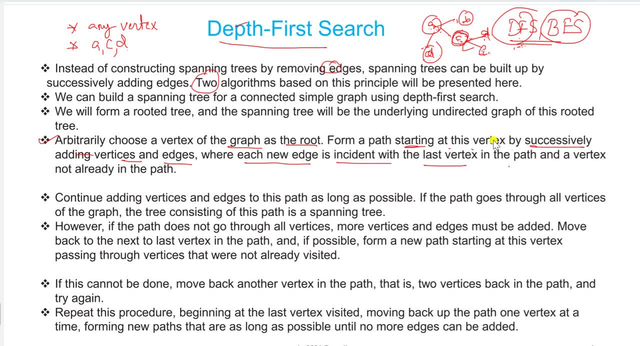 okay here. the thing is, what the vertex that is in the video, if it is there, when you find here that vertex, or should not be already in the path? like this, you are drawing using this. if d again come, already visit this d. oh, so you need not to write it again. okay, if the path does not go. 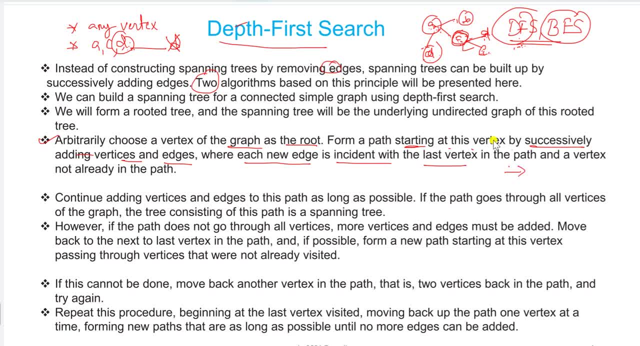 through all the vertices you see here. next condition, here: water. you FIND OUT some path. okay, if the path goes through all the vertices, all the vertices, then the tree consisting of this: what is the tree? is a spanning tree, okay. for example, all vertices through the journey, okay, or a path existing, then we can say that that particular path is nothing but what. 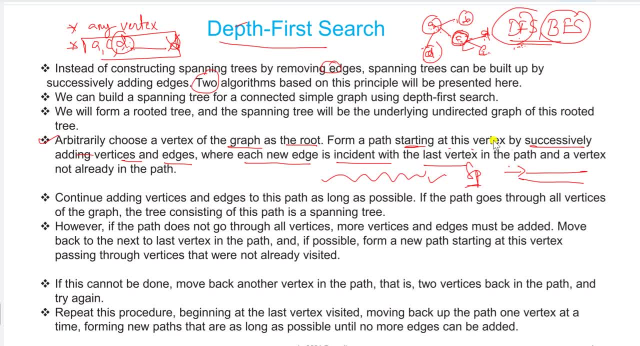 spanning tree. if the path does not go to all the vertices or edges, okay, then it is not a or it is not form the spanning tree. okay, then you have to repeat all the procedure, all this procedure, beginning at the last vertex visited. okay, so last vertex you visited, until this process. 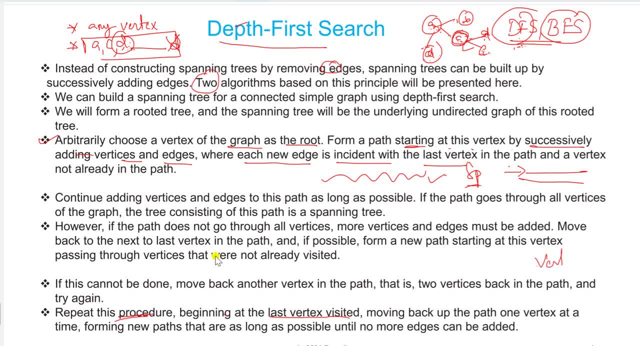 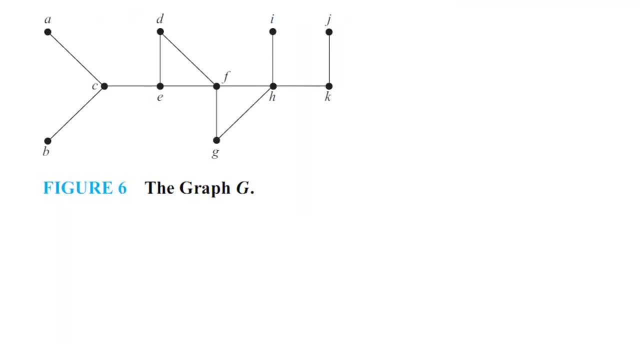 you have to continue this process. if the path or if the vertex is visited, just go back back. tracking process. okay, let us see the example first, then you will get a good idea on this. you will have a better understand after watching the example. now see here. this is my example. 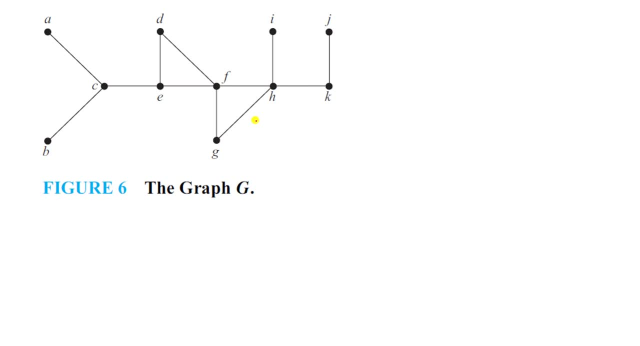 so in this example, you can choose any vertex in order to find out the spanning tree with the help of depth. first switch. okay, i choose f as a my root vertex. okay, so you have to draw f now check, explore this particular vertex. that means what? what are the next visiting vertex? 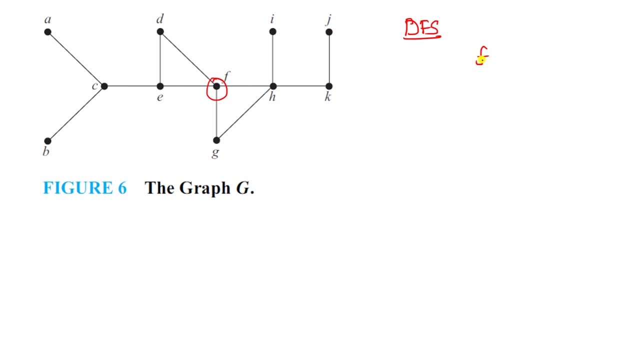 or what are. what is the next visiting vertex and what are the next visiting vertex and what are the next incident of this vertex? you see f have a connection with the or edge with the d and g and e and h. right, how many edges are there? one, two, three, four. okay, among these four you can choose anyone. 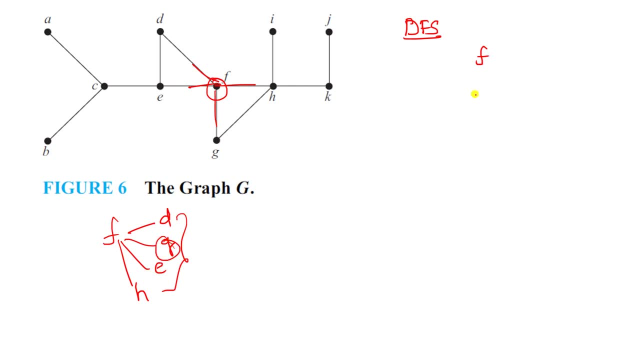 you can choose anyone. okay, i choose g. you can choose anyone. there is no condition or there is no limitation on this. uh, because specific ascending order. choose chase quality. alaim. okay. okay to g. okay now your visiting vertex is what g here? what is the? what is your next vertex? g? 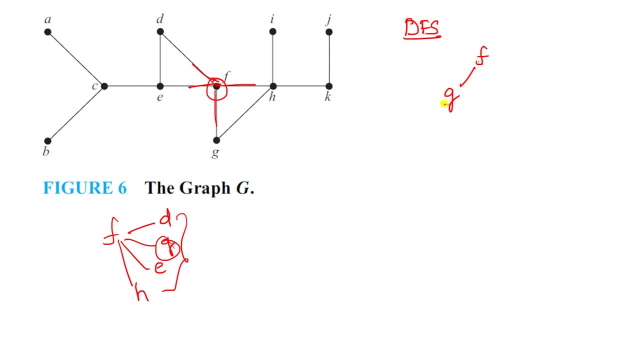 then start with g and explore z. so now check g have how many edges. g have a edge with f and g have a edge with h. okay, now f is already visited, so you should not go to the, you should not write again f, because f is already visited one. okay, now what you have to write: 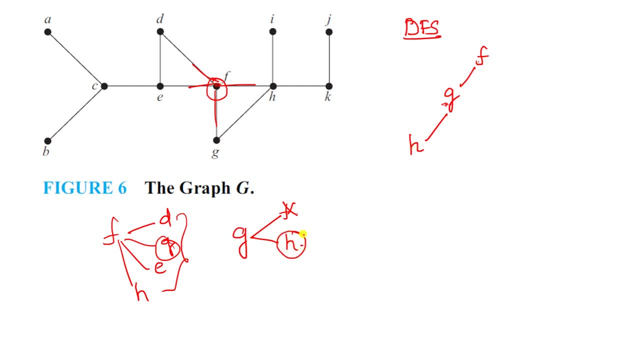 h. okay, so on, your next vertex is what h? and go to h, from f to g, g to h. good, next see h. again here, how many vertices we have h connected with i and k. these two edges are existing with the h. you can take any one, i or k, you can take any one mark. so here i take i. 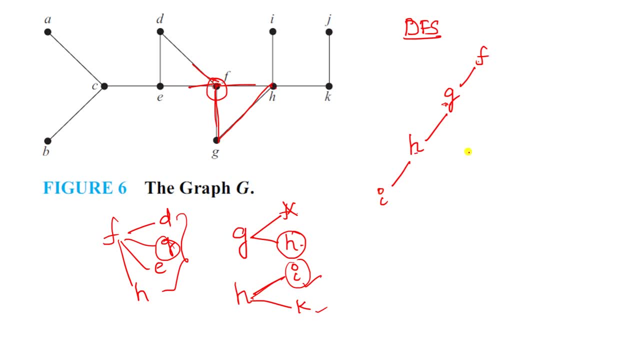 Okay. So see here as a tree: first we have to insert the left part, Okay, And then we have to insert the right part, Okay. Next I and go to the. what is our new vertex? I Explore this. I Does. any H is existing for this, I No, I have only one H. that is H. H is already visited. H is already visited, So no need to write again. as a child of I, Okay. 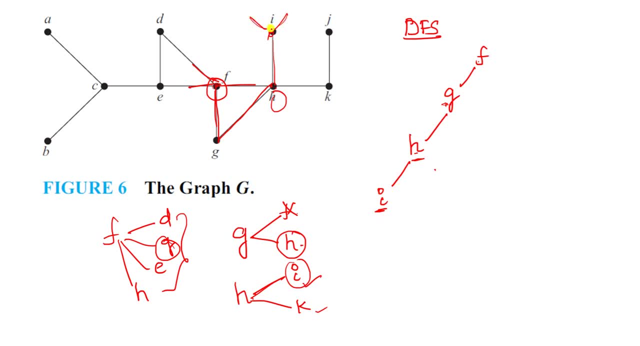 So there is no, there is no edges, particular vectors for this. I So just backtracking to the part. So H. H is already visited. And again check here: H is there. So H have the two parts, Okay, I and K. K is already visited, So you already done this one. And what is the remaining? here, K. Now see where we insert the K as a right child of H, Because we already left child in, left child we insert, Now we insert H. 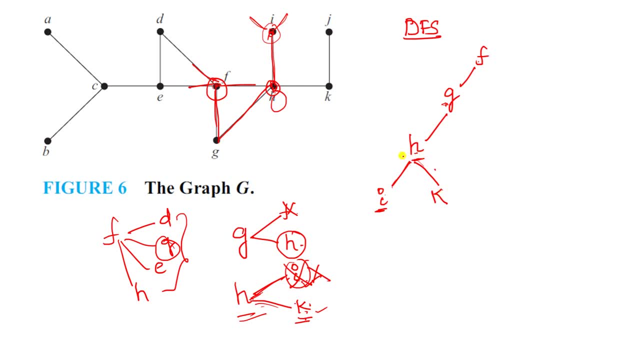 Right part of H, Okay, And what is your new vertex, ma? Now you are in K. Now you are in where K. So check whether any adjacent edges for this K- Yes, K- have a connection with J, And simply only one connection. So just simply you can insert J here, left part of K- Okay, And see what is your vertex Here Now you are here. So J is you need to explore. 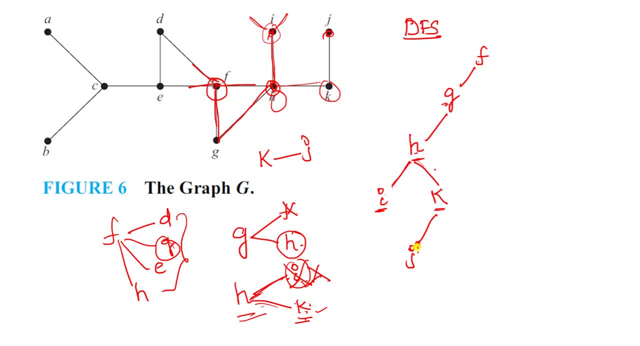 For the J, But still J does not have any incident. Okay, Does not have any adjacent vertices. Okay, The allant edges- kuda mani ki J ninche levo Already only have only one edge, That is K. Already, K is visited, So no need to write again. So, and this step, you have to go backtracking. Okay, So now you visit K- K is already visited- And go backtracking H. H is already visited And check Is still any edges are left with H In. 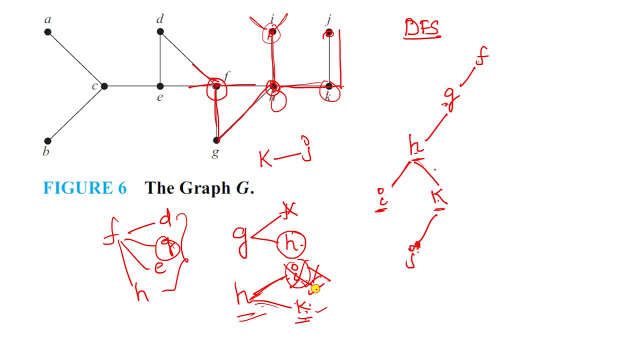 H. we visited I and K already. Okay, You see here, H have the connection with I K, Not only I K. Again, F and G also. H have a connection with I K, F and G. Right Four edges are there still. So I is completed, visited, and K is visited, and F is visited and J is visited, Right, 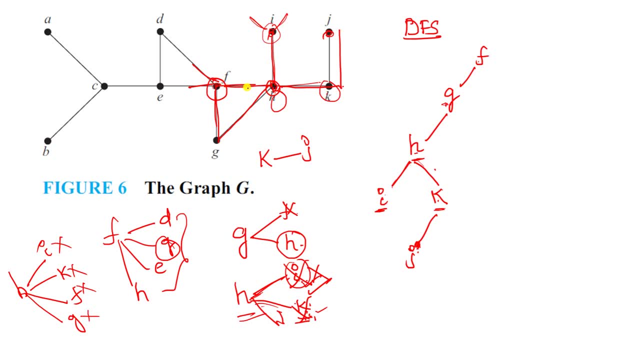 Okay, Now you have to come G, So from K you visit H and next you have to come G. Okay, So here check G. does existing any other We left out with? even we left out with? I have already H and F, So these two are also completed. Next and again backtrack to F, Again backtrack to F And still F have D, Z, E, F In this particular D is a, J. 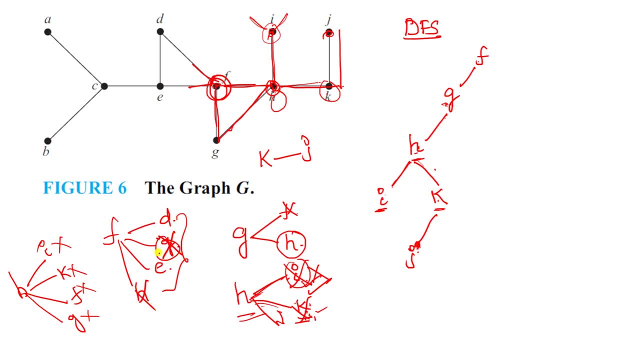 is completed and h is completed and still remaining e and d. you can choose any one of them- e or d, okay. so here i choose d or e, anyone. okay, i choose e here. so come here. e now what is your? explore vertex e. here you need to explore. now check e. e have d and c and f, okay, so see my here. 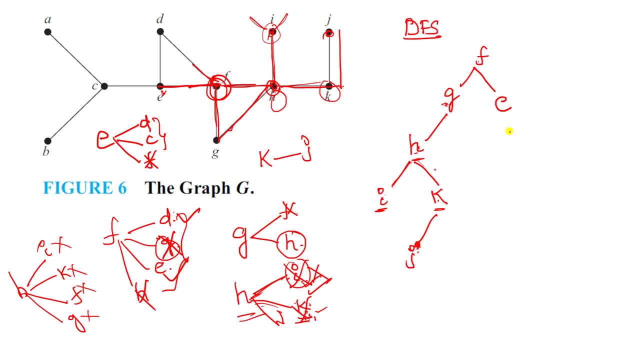 already f is completed and you can choose any one, d or c, so i choose c. so c, i can insert left part. okay, now my vertex, my new vertex, is c and c. here we have c having a and b. still these two vertices are not visited, so i can take any one of them, so i choose a. okay, 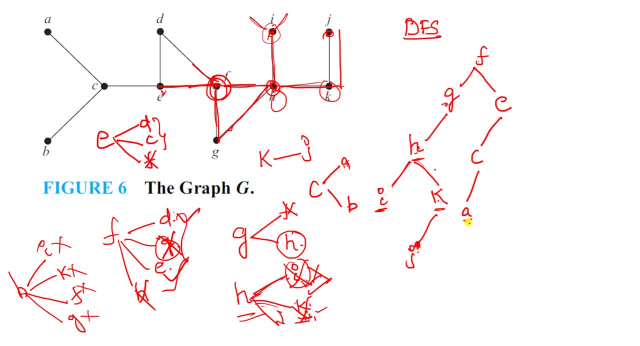 and now my new vertex is a. here a does not existing any new path or any edges, only it has only one part, that is c. so c already visited. so i just go backtracking, okay, backtracking. and then c is: a is finished, right, a is completed. now what is there? b only there. so 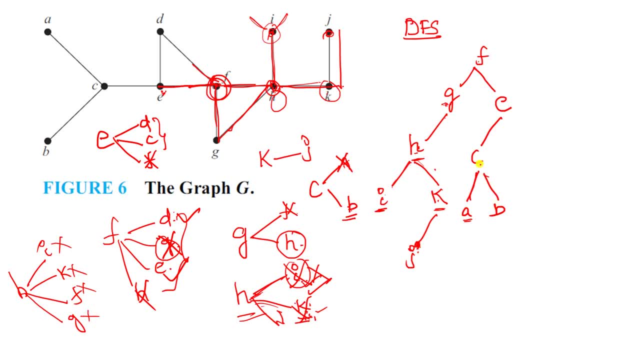 a and b. still, these two vertices are not visited, so i can take any one of them. so i choose a, B- Okay, And go back to C, Because B does not have any other edges Right, Go back to C And from C, where we have to move E- Okay, And E And check E. Where is the E? C is completed, Now only. 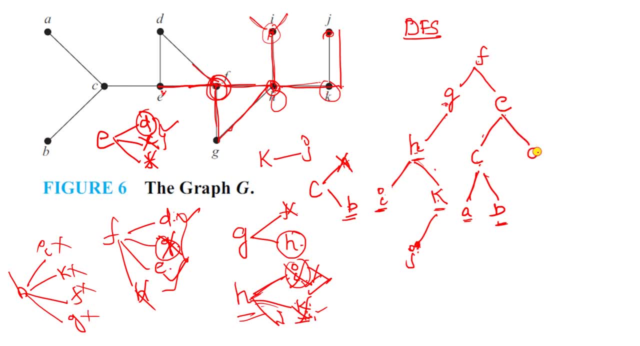 what is the vertices left with E? That is D. Okay, This is my spanning tree for this particular graph Like this, you need to find out spanning tree with the help of depth first set. Okay, What is the process, ma, The first step you need to take. you can take or you can choose any vertex as a. 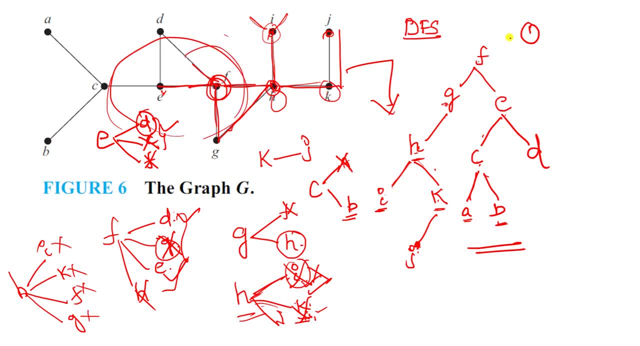 root node from this graph: Okay. In this graph you can take any vertex as a root node. Okay, And the second one: explore that particular vertex. Explore, Explore means what? here You can visit any new node. You can explore any new node. You can explore any new node. You can explore any new node. 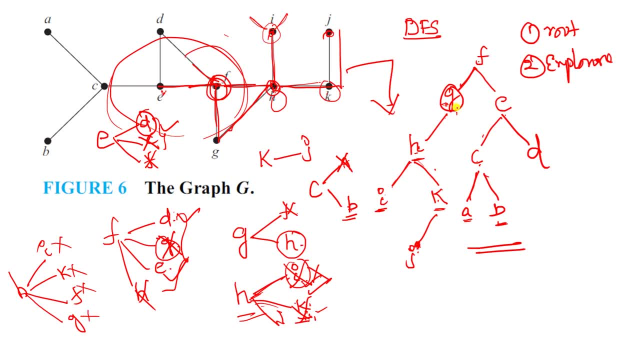 Start with this vertex. Okay, What is the next incident vertex of this particular G? Okay, That is a thing. And the third, third one is what You have to check: whether that particular vertex is already visited or not. Okay, If it is already visited. if it is already visited, then you should. 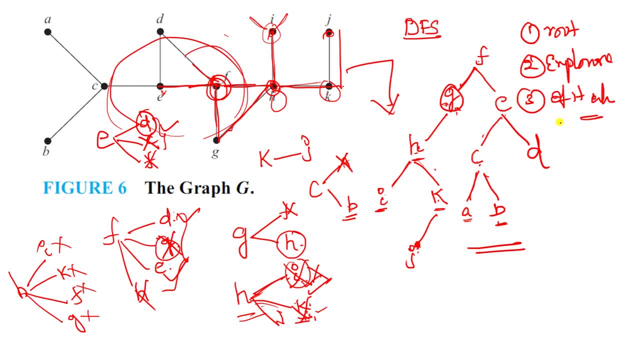 not take Okay. If it is not visited, then you can take Okay And then explore it. That is the next step. Okay, You have to do this process Until you reach the last vertex, or until you visit all the vertices in the graph. Okay, This? 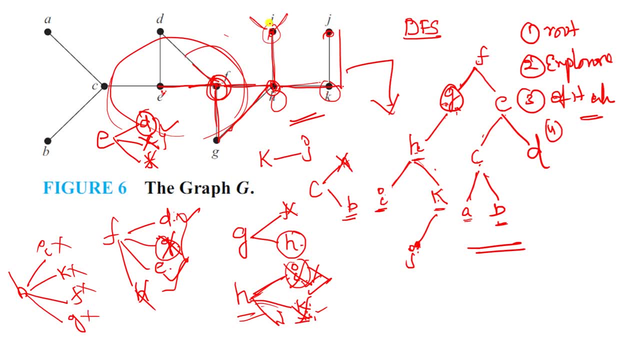 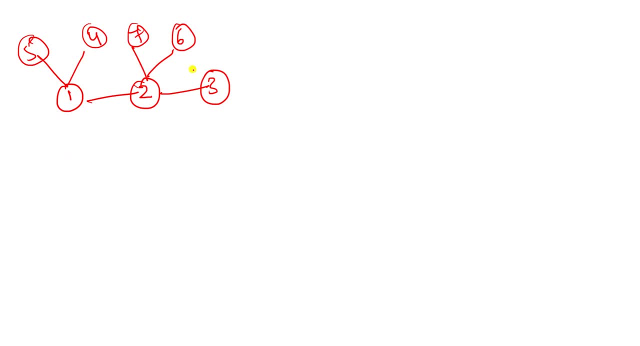 this is simple, ma Very, very simple. See this another example here In this particular graph. So which element we can choose? Can we choose two as a root node? Okay, So I want to construct the spanning tree from this particular graph with the help of DFS algorithm. Okay, I am going to. 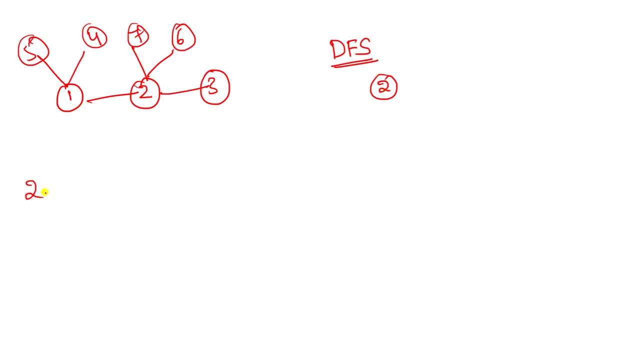 choose two as a root node. Okay, Now write down two. What are the edge vertices for this? One and seven, and six and three. So choose any one of them. Okay, I choose one, So I insert one here. 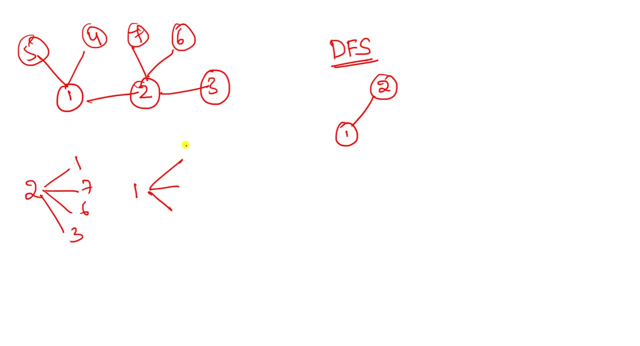 Now write down what are the edges of the one. One have five and four and two Right. So among these two is already visited, So you can eliminate this one And next remaining five and four. I write: I choose five. 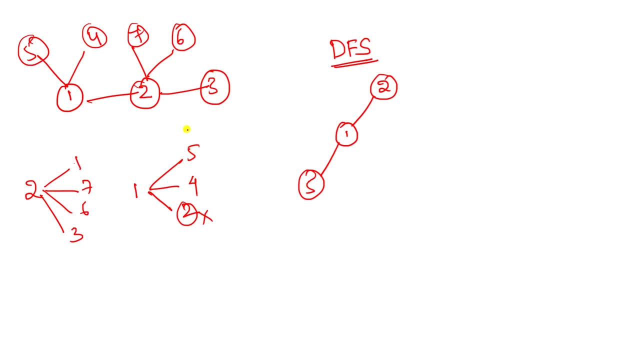 As a another vertex: Okay, I visit five. Okay, From one I visit five And next I come back to one, because there is no edges, are there for five? Okay, So I come back, or backtracking, to one, And now 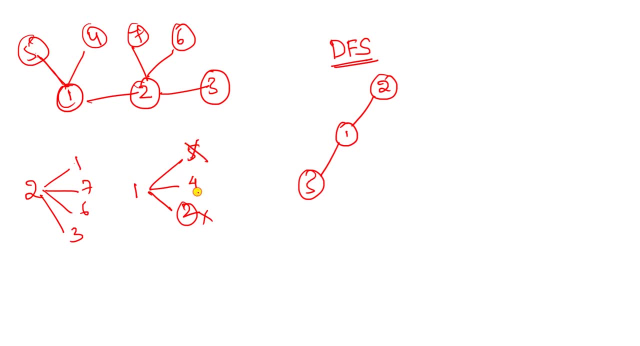 still there is a. one vertex is remaining in the one, that is what? four. So I need to insert the four at the left part of one. Okay Now, So four is also completed. So from this, from this level, one node is completed. One visited all the vertices Right. Two: One visited to two. One: 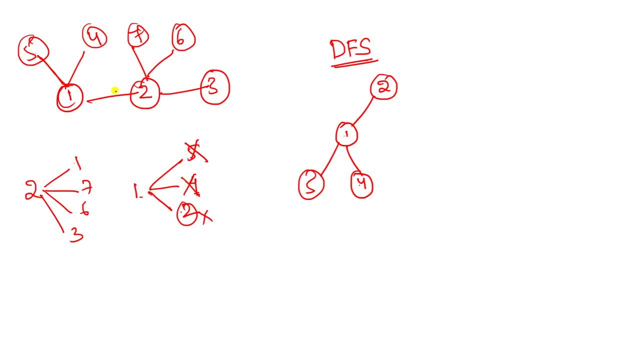 visit four. One visit five, Right, ma, And see the next one. I come back to go back to the second vertex. See here, Back to backtracking to this particular vertex. So here two have a one, seven, six, three. So one is completed And the remaining what are there? Seven and six and three. 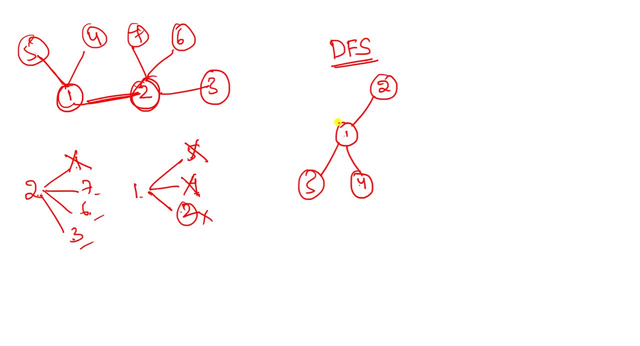 Right, So I choose any one. Okay, You can choose any one. So I choose seven. Okay, You can choose any one, I choose seven. So you see here, seven does any vertexes adjacent vertices is existing for this seven? No, Right, Because seven have only one vertex, that is. 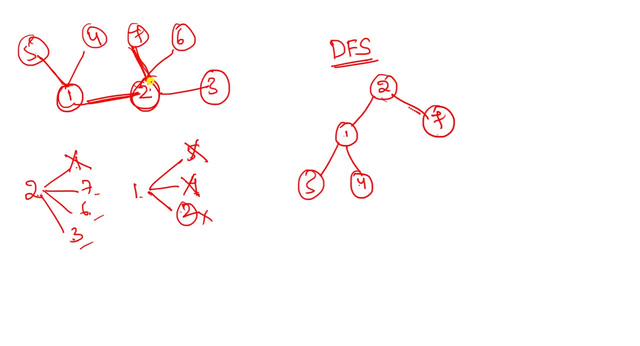 two. So two already visited. So backtrack to two, And seven is completed here. Now what is the vertices? we have Three, So I insert three like this, And next three does not have any other edges. So I backtrack to the tree And now you can insert. 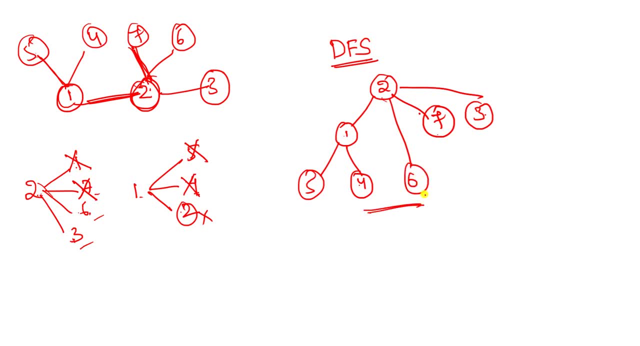 another one, that is six. Okay, Like this, you can construct the spanning trees. For the same graph, I choose one as a vertex. Okay. From the same graph, I choose a one as a root node, For example: Okay, So what is the next vertices can we choose? Can we, can we choose one half? 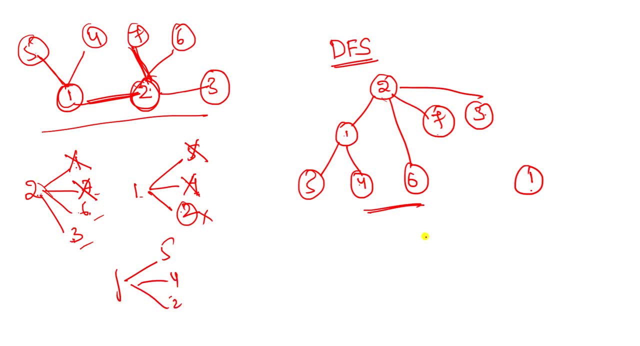 five, four, two ma. Okay, So I choose two as an another vertex. So here two inserted at here. Now we are in two. Right Now explore this two. So write down what are the edges. 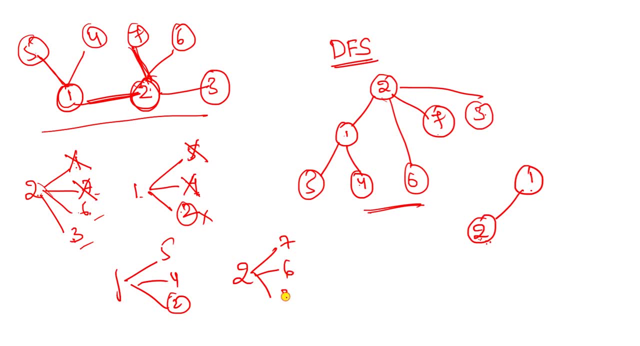 for this two. Two have a three edges, called seven six three. So among the seven six three, I choose three. Okay, So three is inserted in the left part of two And next one. now we are here. 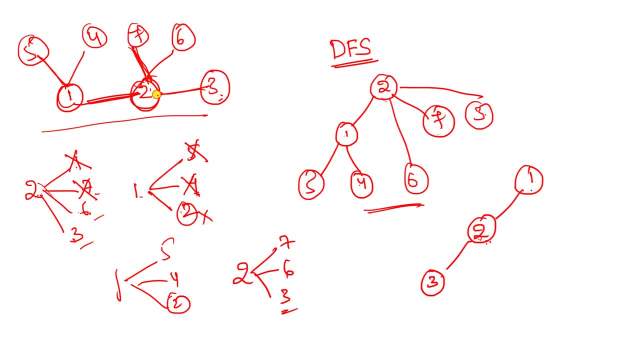 Okay, So there is no specific edges for this, So we backtracking to the two. Okay Again, we are now here, So two have edges with seven, six, three. So three is already completed and the remaining seven and six. So in the seven and six we can choose anyone, Right? 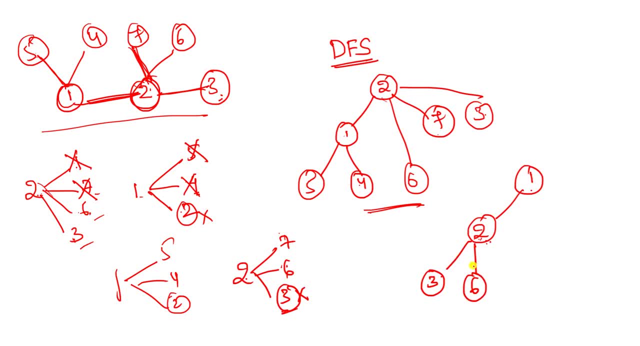 So I can choose here six And the same same, here six does not existing any other edges, irrespective of two. Okay, Only it has the two, that is edge with two. Okay, So we are here. So again we are backtracking to the two and I visit seven. Okay, Again here seven. 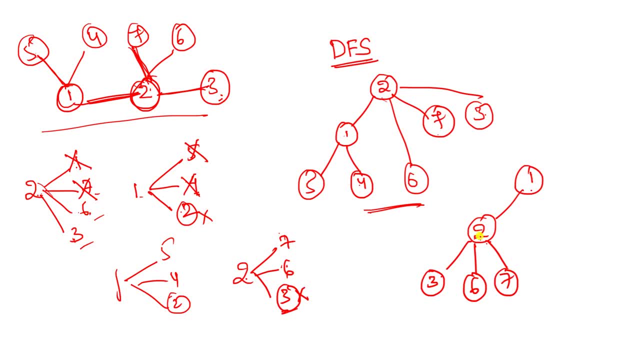 does not existing any adjacent vertices, So we backtrack to the two and from here to two, all the vertices is completed. Okay, All the adjacent incident vertices are completed. Now come to the one. Okay, See backtracking to the one Right. So in one have five four. 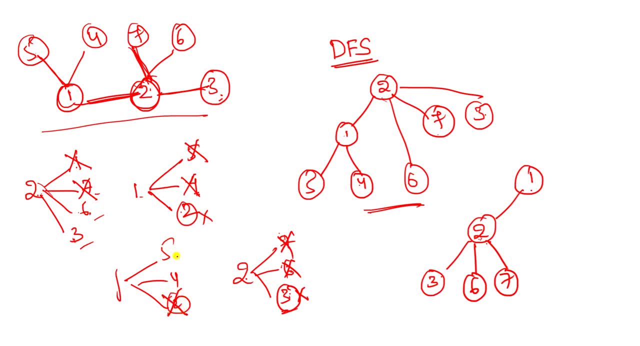 two. Two is already visited, So no need to write it again. and the remaining, what are there? Five? four, three, four, three, two. Two is already visited, So no need to write it again. And remaining, what are there? Five? 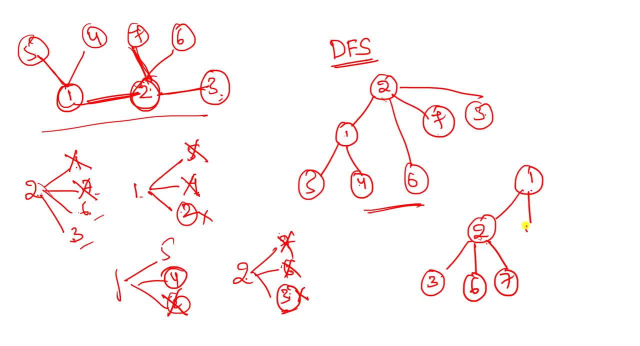 and 4. okay, you can choose 4. so insert 4. so does any edges, adjacent edges? is there for this 4? no, so you can backtrack to the 1 and again the rest. only one edge is pending there, that is 5. check whether all the elements, all the vertices, is there or not. yes, all the vertices is there. 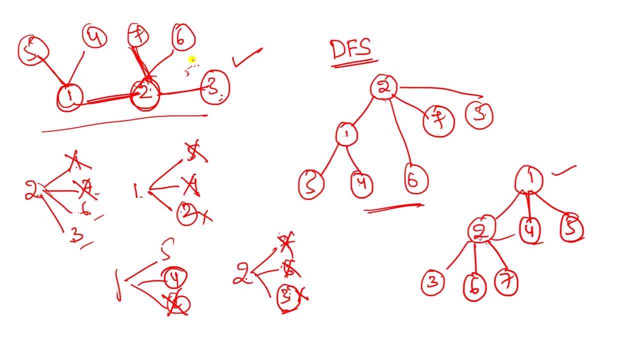 what are there? what are the vertices? is there in this particular graph? all those vertices are there in this graph. okay, like this, you can construct any number of spanning trees for a graph. okay, you can choose 1 as a root node, or you can choose 2 as a root node. you can choose 3 as a root node. 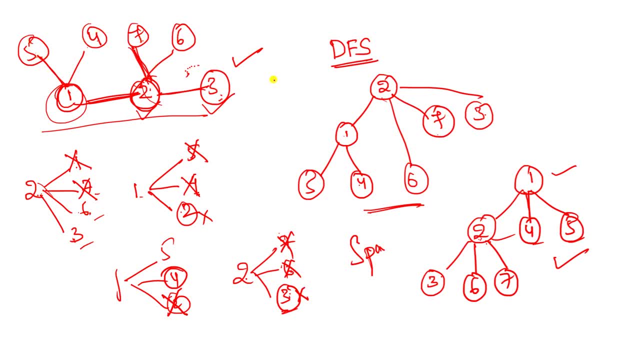 you can choose anyone. 5, 4, 7, 6 among the 7, you can choose anyone as a root node. okay, there is no any limitation to choosing the root node. that is the best case in the dfs. okay, in case in examination, if they ask, start with the root node. 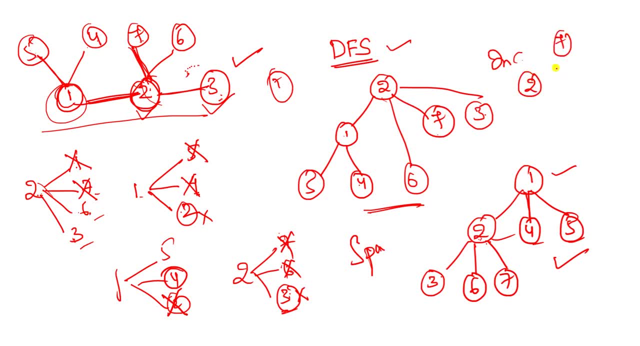 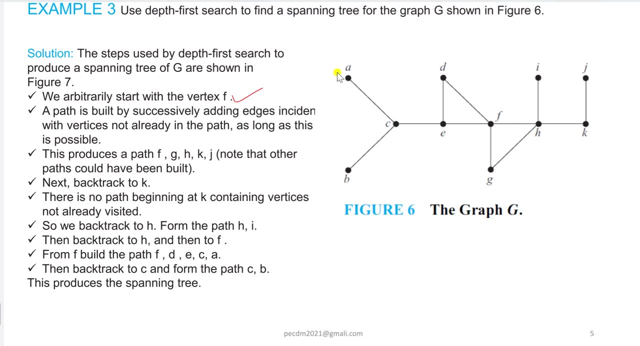 2 or start with the root, node 7, then you have to mention it as it. you have to take it at the 7 right, otherwise you can take anyone. okay, hope you understand. so see here the here in this notes i gave this um. you have to write um all these particular steps, ma in examination, because 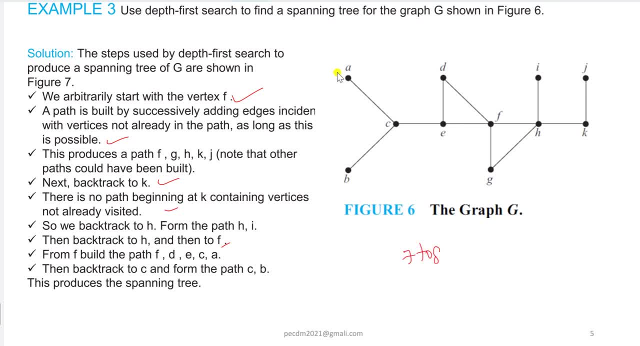 this is a 8- 7 to 8 marks question. okay, it is a 7 to 8 marks question. okay, you cannot directly draw the graph or you cannot directly draw the trees. okay, you should not directly draw the trees. okay, now give you a graph and find out. first you need to write the definition of the spanning tree. okay, this is the structure of writing the answers in exam. okay, first you have to write definition of spanning tree and then there should be algorithm for this- DFS and BFS- a simple algorithm, how we can construct. 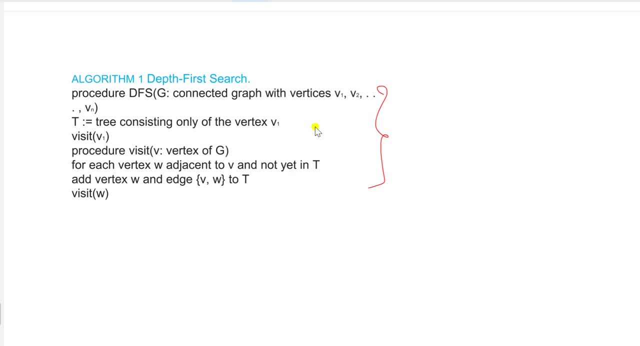 you see, this is the algorithm for DFS. so first, G should be a connected graph with a number of vertices and a tree consisting only one of the vertex V1, and we have to visit that particular vertex and each vertex we have to write the next adjacent vertex. okay, that is the process. we have to go, we have to do right. so how to write a depth first search algorithm? if they ask in examination for 8 marks, first you need to write the definition of spanning tree. 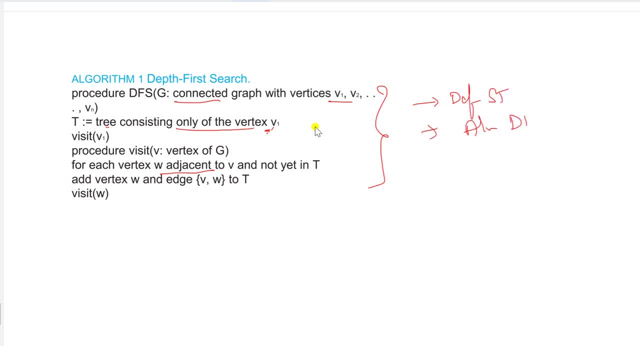 and then write down the algorithm for DFS. if they ask BFS, BFS algorithm- right. if they ask DFS, DFS algorithm, right, okay. and then write down that graph. okay, a specific graph. first, check whether that graph is a connected one or not. compulsory. they will give the connected graph only, for connected graph only. we can connect the spanning trees, right. so draw that graph and write down the steps. okay, what you choose, the root node. after that, what is the? you have to explain the. 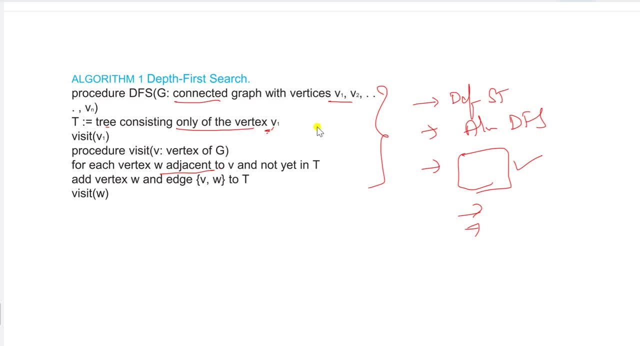 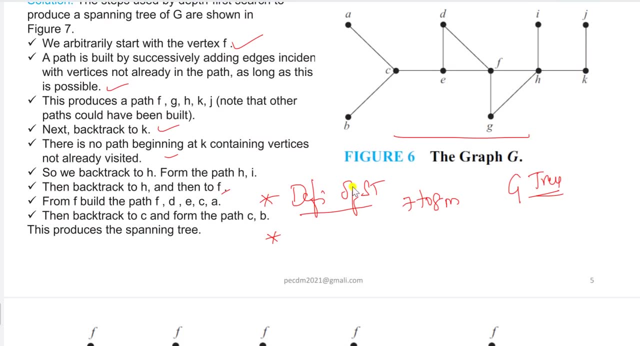 exploring vertex. each and every step you have to write in detail manner. okay, so that procedure I have already provided in your notes. right, so how we can deal: first we have to visit the particular notes and next you have to visit like this and backtracking to the k. okay, so each and 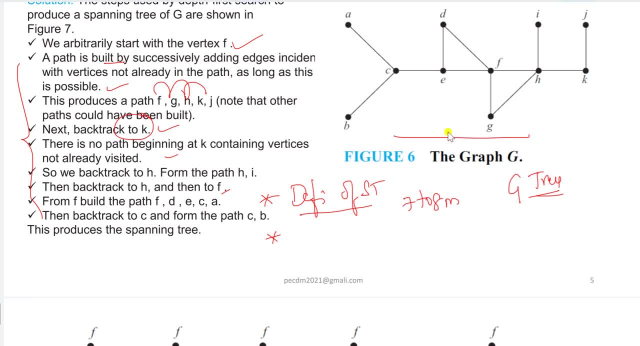 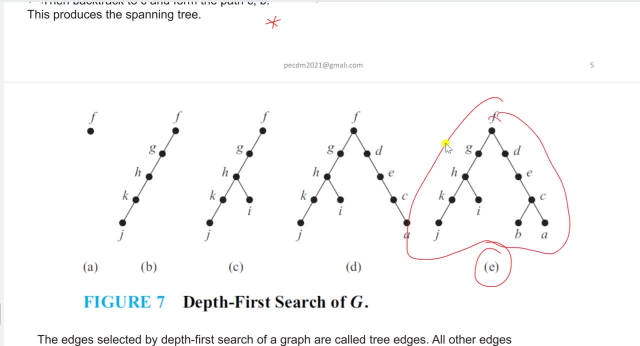 every step you have to write in detail in the exam so that you will get good marks. and finally, this is your spanning tree. this is your spanning tree if f is a root node, okay. so finally, you have to explain that this is the spanning tree, right? so this is about depth first. 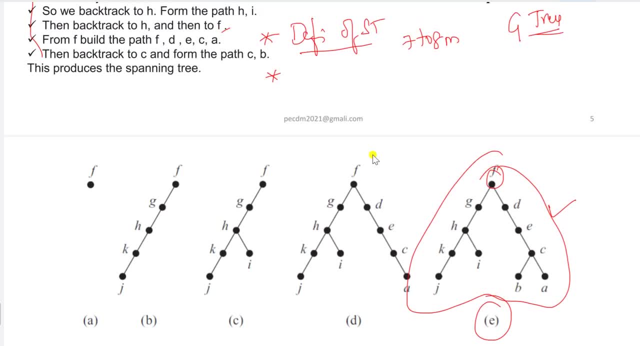 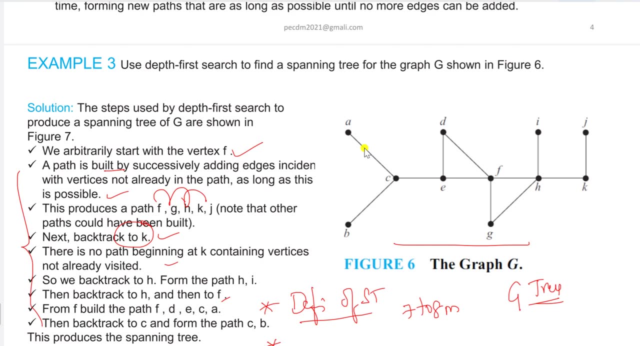 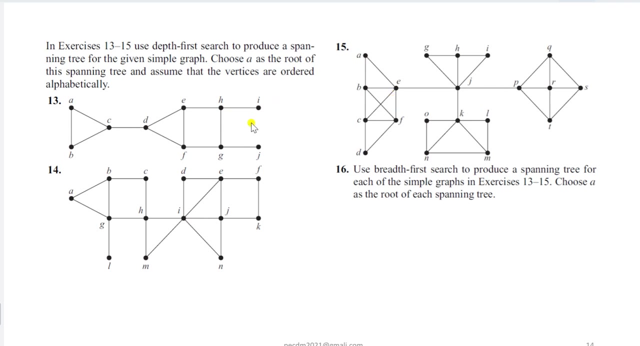 stitch and the next class. I will explain: breadth first stitch, how we can find out the spanning tree with the help of breadth first stitch. okay, that is also very simple one. hope you understand this concept You see here. please try to make it down right. try to do depth first stitch and find out the. 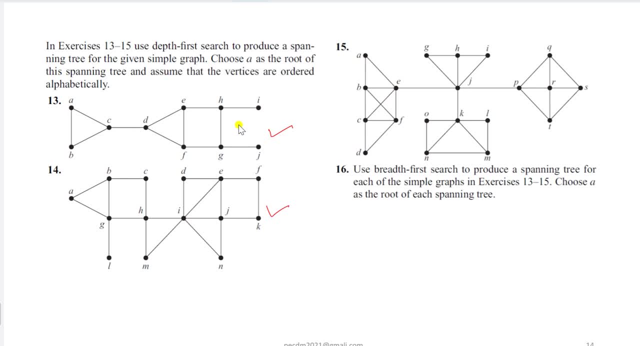 spanning tree for this particular graph and find out the spanning tree. find out the spanning tree for this. all these graphs, okay, next class I will discuss each and every one. okay, next class I will explain this, but you just try now. okay, and see here what they ask.